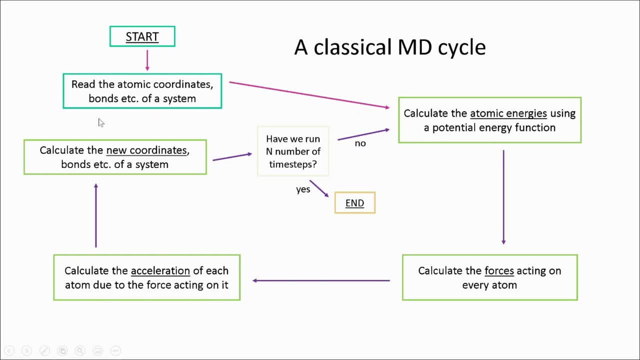 information of your system, as well as any initial velocity. Then the atomic energies are calculated using our potential energy function. From these energies, the force acting on each atom is computed. The forces can be used to calculate the acceleration of each atom in a particular direction. These are then used to generate new coordinates for 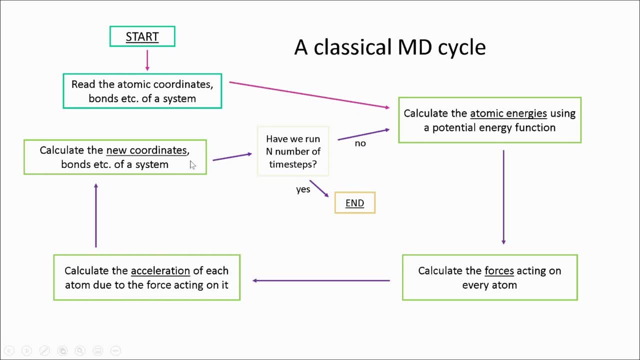 each of our atoms, as well as their new velocities. The program checks if n the specified number of times has elapsed. If not, the program repeats the same process, repeats the cycle and computes new coordinates for the system. This cycle is repeated until 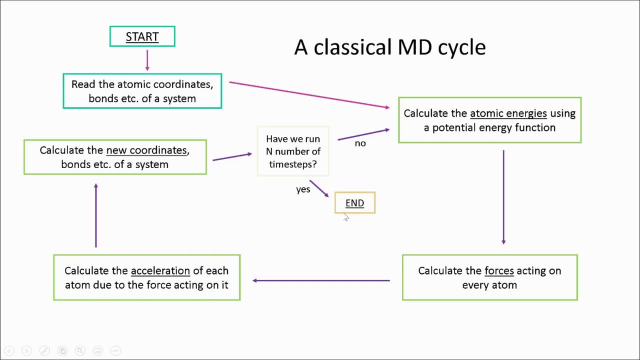 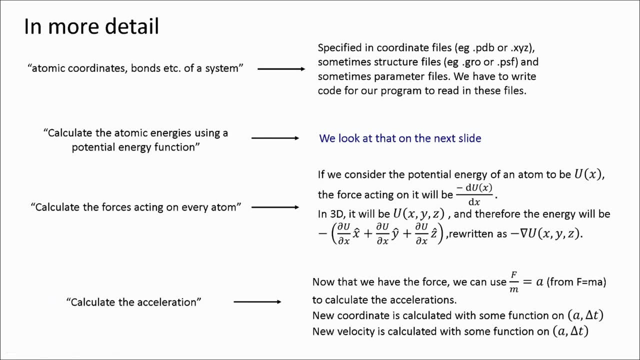 n number of timesteps has elapsed, at which point the program will write all of its computed data in an output file and terminate. We can then post-process this file and look at our results. Looking at the system in more detail, the system information is first specified. usually, 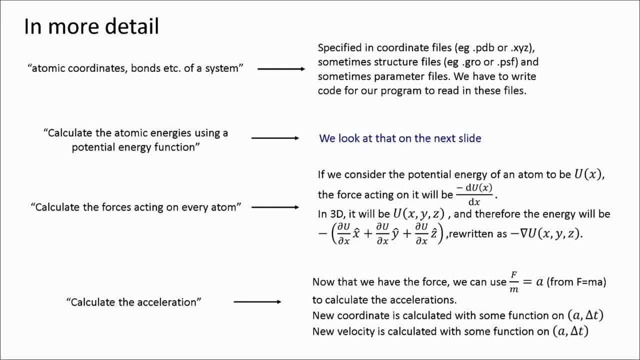 in a group of files – a coordinate file, such as a PDB or XYZ file, a structural file, such as a PSF or GROW file, and usually a force field parameter file, such as a PRM file. Most molecular dynamics simulation programs use an input script where you specify the 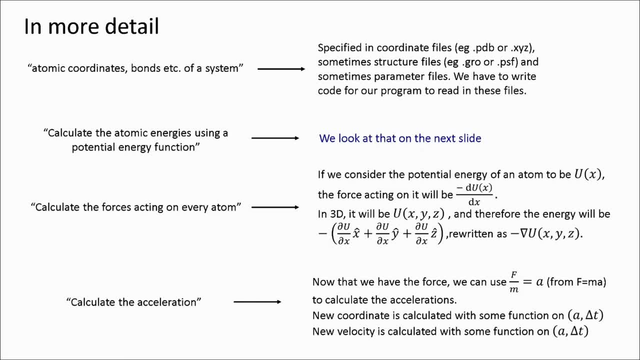 names of these files or even copy the file information into the actual input script. We will look at the energy function in our next slide. Having calculated the energy of an atom- let's call it u of atom x- we can see that the force acting on it will be the negative. 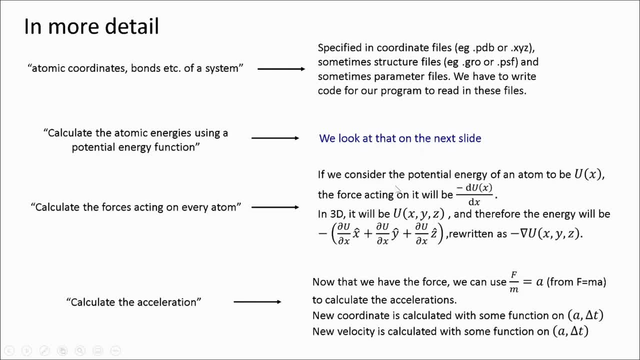 derivative of u of x. Seeing as our atoms are not one but three-dimensional, the force will be a combined partial derivative of each of the principal axes. Don't be intimidated by the math. it's just splitting up the derivative into three parts that each deal with one of the three. 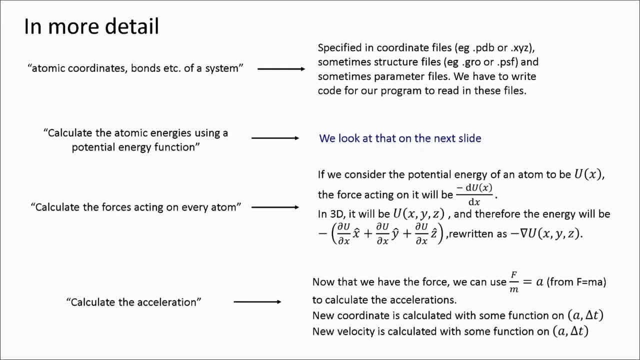 dimensions to then get a three-dimensional force vector. Finally, we can use Newton's second law to calculate the acceleration acting on each atom. As you can see here, this will also depend on atomic mass and therefore the element that each atom is representing. Using the acceleration. 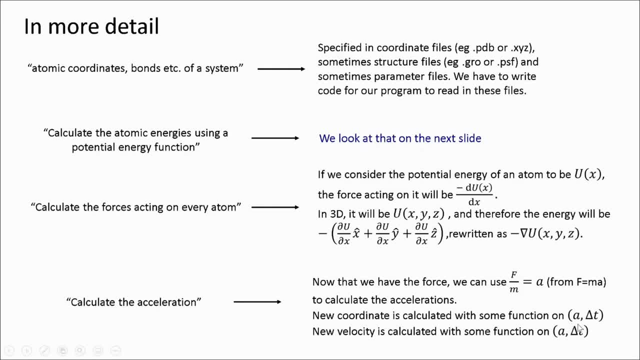 and an already specified time step duration, for example one femtosecond per step. we use some kind of function to calculate our new atomic coordinates and velocity. We then represent the acceleration acting on each atom, and we can use the acceleration acting on each. 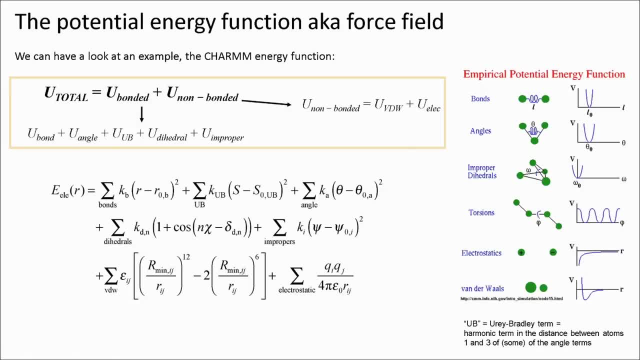 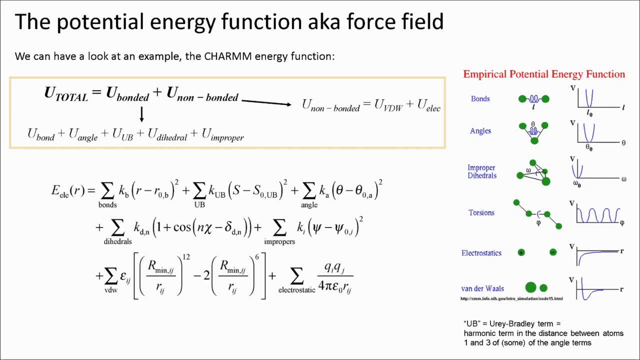 at an example such as the charm force field. Here we can see that, according to the charm force field, the total energy of an atom consists of its energy associated with the bonding and the non-bonding interactions. The bonding energy is itself composed of the sum of the energy. 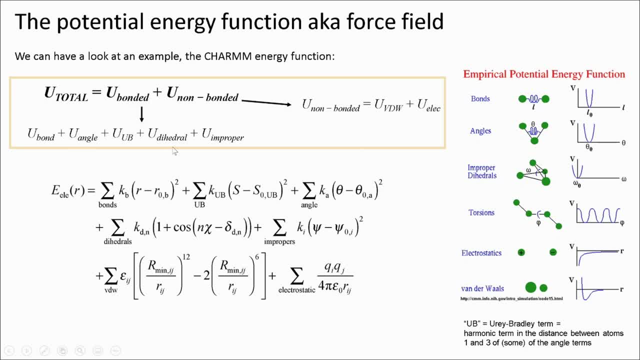 associated with the atomic bonds, the atomic angles, atomic dihedrals and atomic improperly. You may also wonder what the UB term stands for. This is a term that is found in the charm force field, specifically called the Urey-Bradley term, and is described as the harmonic term in the distance. 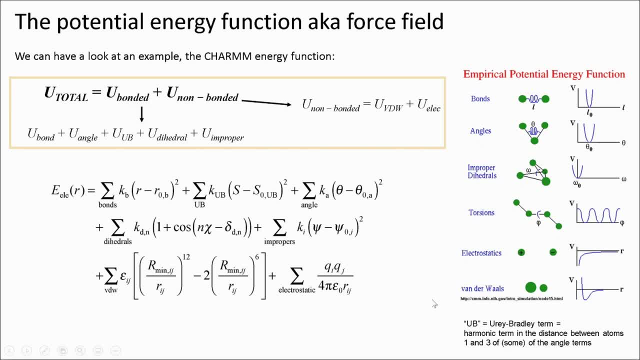 between atoms, one and three of some of the angle terms. The way that these manifest themselves is that, depending on the distance between two bonded atoms or the angle between three atoms or four atoms in an improper or dihedral, different energies will be assigned. 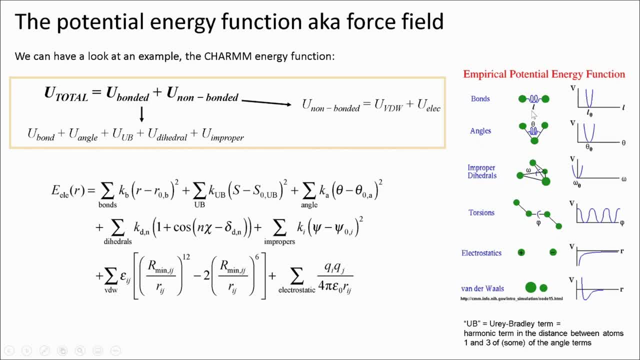 For example, if we look on this chart to the right and we look at the bonds term specifically, we can see that there is an optimal length between two atoms and depending on the length, a different energy value will be added. Keep in mind that capital E, V and U are all used. 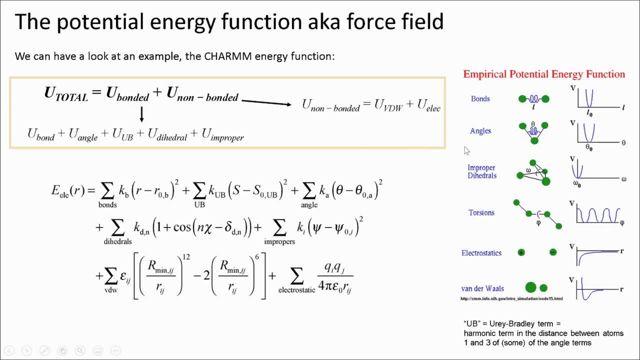 to represent energy and are just different terms for the same thing. The same is true for the non-bonded energy comprised of van der Waals interactions, also sometimes called the Leonard-Jones term, and the electrostatic interactions which happen between charged particles. All of this combines. 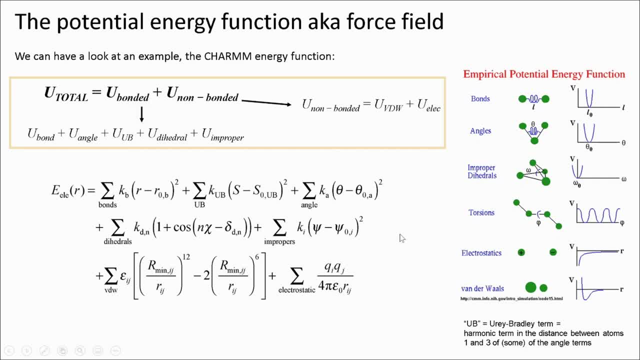 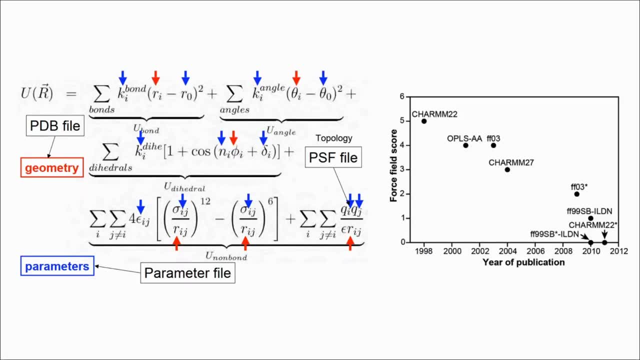 into one equation that we can see here, where each contributing energy is given with some variable. that are all taken from our input files. Looking at the slightly older version, the charm force field equation, we can see where the different values from calculating the energies 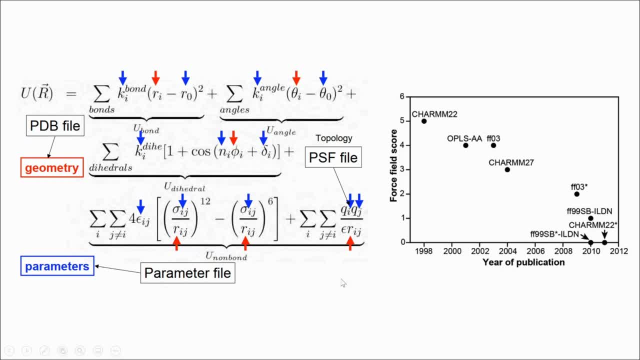 come from. We can see that variables with red arrows come from PDB geometry, aka coordinate structure, and variables with blue arrows are taken from the parameter file, while the two variables needed for the electrostatic energy term are taken from the PSF structure. 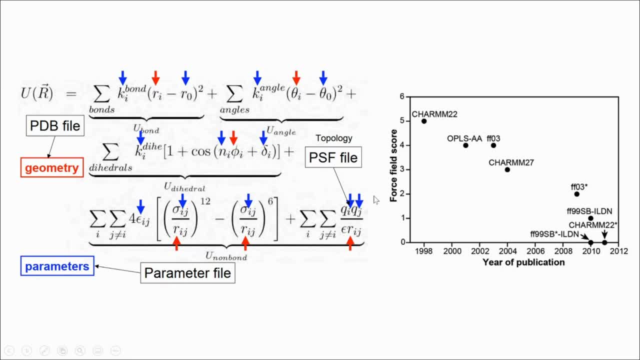 file. This is why it is important to have accurate values in your coordinate structure and especially your parameter file. Even a small change in these could massively affect the behaviour of the simulation. On the right we can see a graph that has rated different force fields on their accuracy. a lower number, signifying greater agreement with experimental data. This is because the two variables are not the same and therefore they have different values. For example, if you look at the graph on the right, you can see that the two variables are the same, but 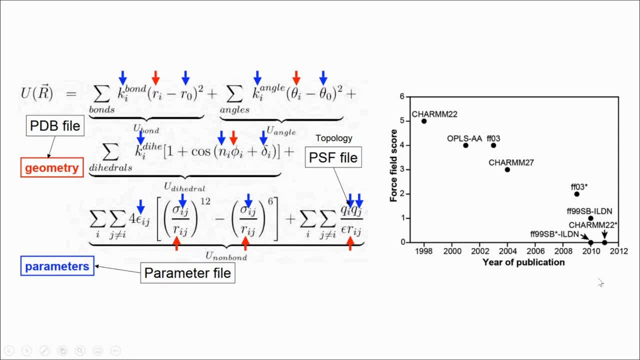 they are not the same. It is also important to choose the right force field for your simulation. Some force fields, such as charm or OPLS, are specifically designed for biomolecules, while others are better at simulating crystallographic or small molecule systems. 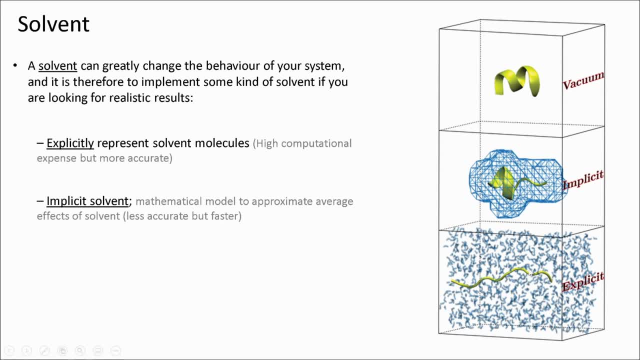 Now that we have gone over the basics of molecular dynamics, let's have a look at a few more things that we are going to want to keep in mind. The first of these is our solvent model. The presence of a solvent greatly changes the behaviour of a system, and actually changes the behaviour of the system. For example, 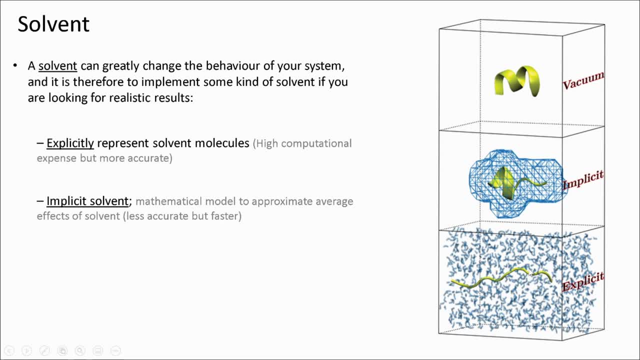 the presence of a solvent greatly changes the behaviour of a system and actually changes the behaviour of a system. The presence of a solvent greatly changes the behaviour of a system and, as such, it is important to consider solvent models if you want to get the results that 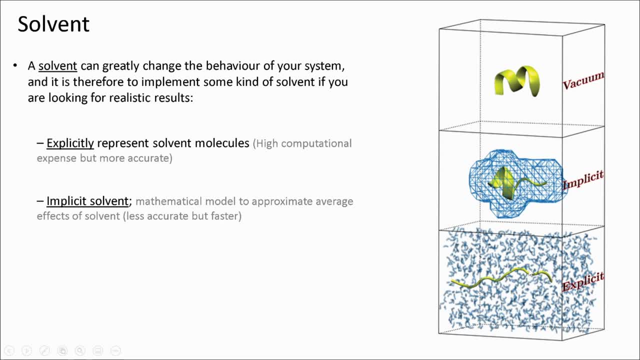 agree with the experimental data. The simplest thing you could do is ignore the solvent. however, this will often lead to inaccurate data and will greatly change the properties of the molecules in our system. The next step up is an implicit solvent model. This is more computationally expensive and 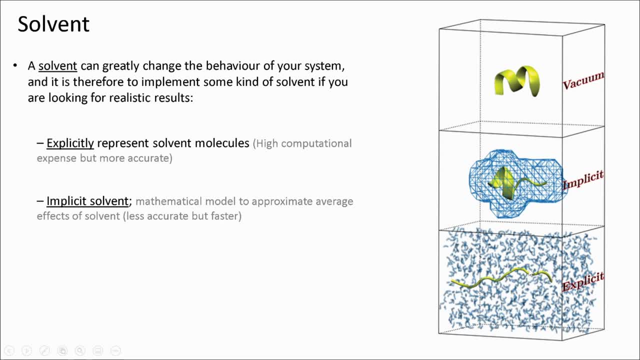 we still aren't simulating actual solvent molecules, but instead our program imagines that there is a sort of solvent force that permeates our system. Finally, we have the explicit solvent model, which is the most computationally expensive but also the most accurate one. We actually fill up our system with solvent molecules. 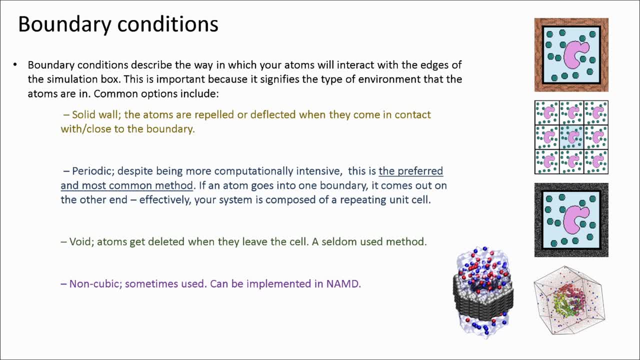 and do molecular dynamics calculations on them. Another important thing to consider is our boundary conditions. These will govern the behaviour of our molecules when they come in contact with the simulation box, edges or boundaries. Common approaches include solid wall, having a solid wall that deflects or 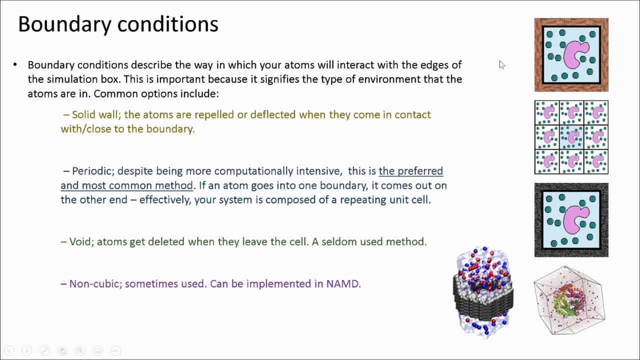 repels atoms when they come in contact with a boundary Periodic- by far the most common method, as it most closely resembles real life. Periodic boundary conditions mean that if an atom goes into one boundary, it comes out of the opposing boundary. We can think of 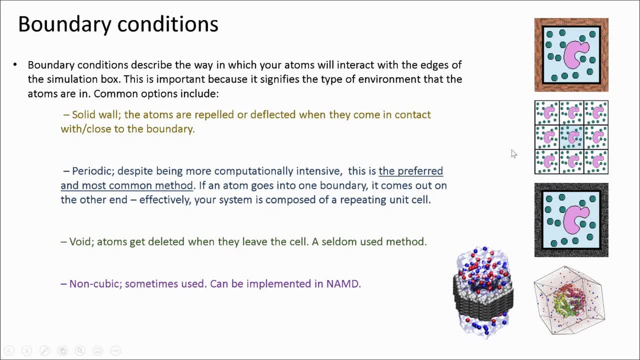 this as an ever repeating unit cell of our simulation space. Some simulation methods delete the atom or simply crash when an atom goes into a boundary. Sometimes we even use a non-cubic simulation space, such as a hexagonal, spherical or cylindrical shape. 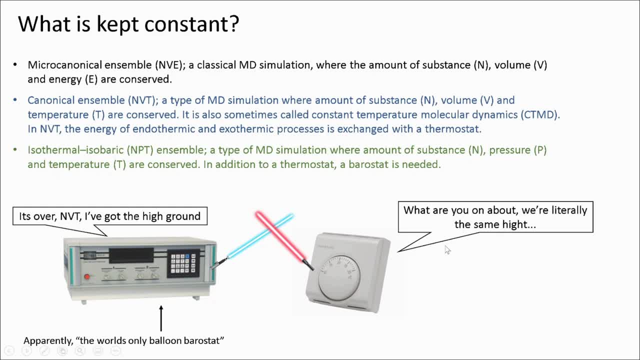 There are also simulation protocols that can keep specific things in our system the same by altering different variables. You could refer to classical molecular dynamics simulation as a microcanonical ensemble, or NVE for short. The NVE stands for the things that we will keep constant: The amount of substance, the amount of time, the amount of time we have. to keep those constant. The NVE stands for the things that will keep constant the amount of substance. the amount of time that we need to keep constant the amount of time that we need to keep constant. the amount of time that we need to keep constant the amount of substance. 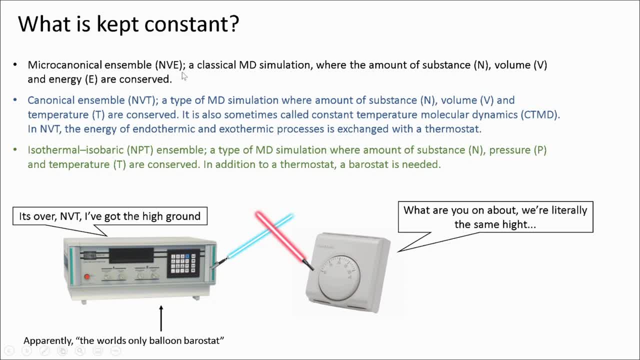 the volume and the total energy. Another method is the canonical ensemble, or NVT for short, where the amount of substance, volume and temperature are conserved, which is why it is also referred to as constant temperature. molecular dynamics. We can refer to the 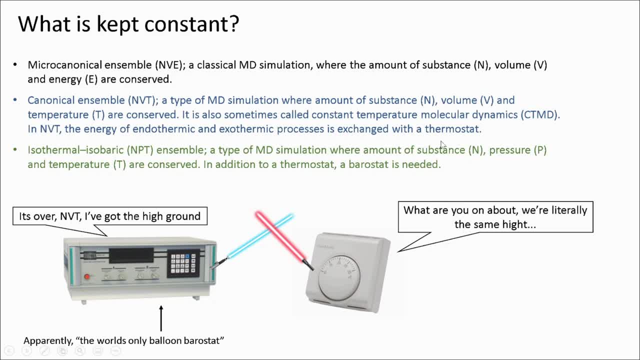 implementation of this as a thermostat, because the temperature is kept constant. The isothermal isobaric ensemble, referred to as NPT, keeps the amount of substance pressure and temperature constant, In the same way that we had a thermostat to keep the temperature. 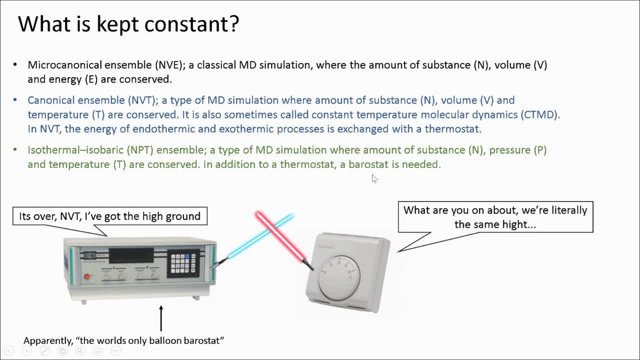 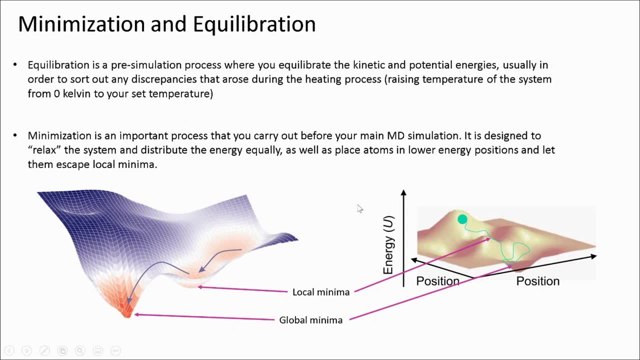 constant. we refer to the method used to conserve the pressure as a barostat. Two more terms that are used very commonly in the world of molecular dynamics are minimalisation and equilibration. Equilibration is a process that we carry out before our main simulation, where we equilibrate. 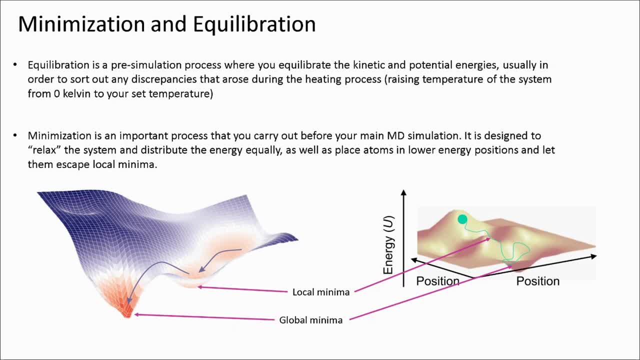 the kinetic and potential energies across the system, usually to sort local groups of high energy or energy sources. This is a process that is often used to calculate the energy for any other unnatural phenomena in our system that usually get created during the heating process, where molecules are provided with energy and therefore the so-called temperature. 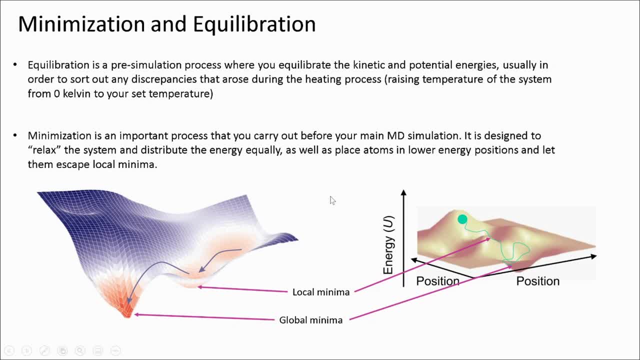 of the system is raised from zero kelvin to our specified temperature. Minimisation is an important process to carry out before our main simulation. It is designed to relax the system, distribute the energy around the system and get as many atoms or molecules out of their local minima into global minima.